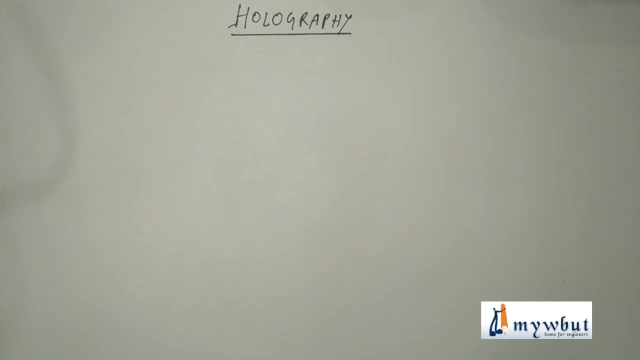 and reproducing a three-dimensional or 3D image of object without the use of lens but using the coherence properties of laser beams. So that is why in the syllabus holography is given just after laser, because after studying the properties of laser we have to study the uses of laser and the 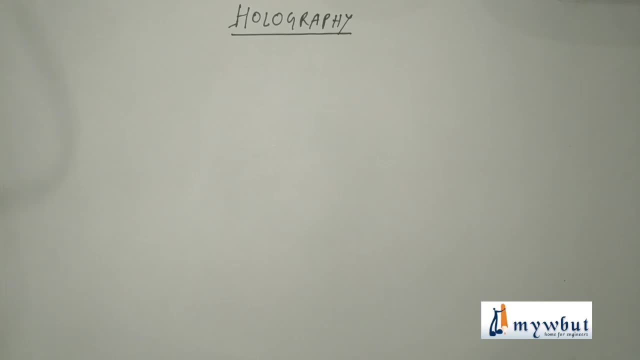 very modern and scientific use of laser is holography. So let us now see. what is this? Holography is a method for recording and reproducing a 3D image, but it doesn't use lens. as I have already said before, It depends on the principle of interference of an. 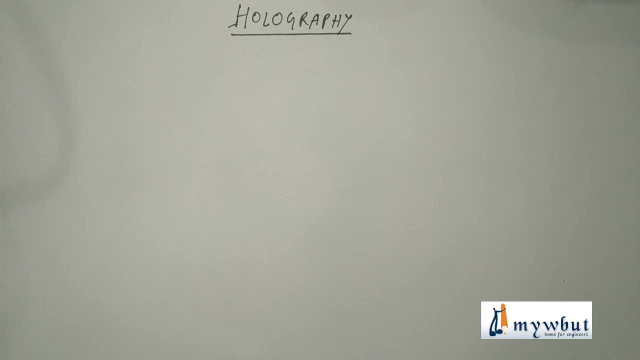 object with a reference wave of highly coherent in nature. So in holography, both the phase and intensity, that is, amplitude of the light waves, are recorded on a film, and the light waves are recorded on a film And when the photograph is viewed it shows a 3D image of the object. Such a 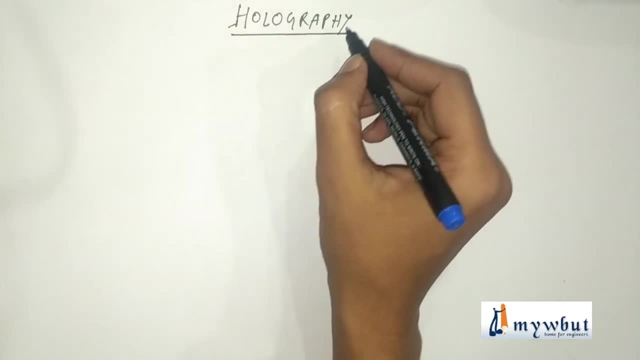 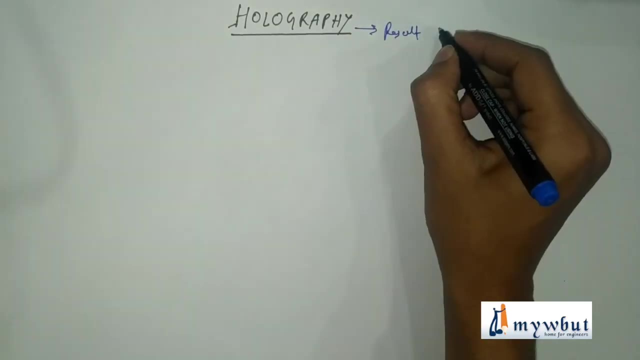 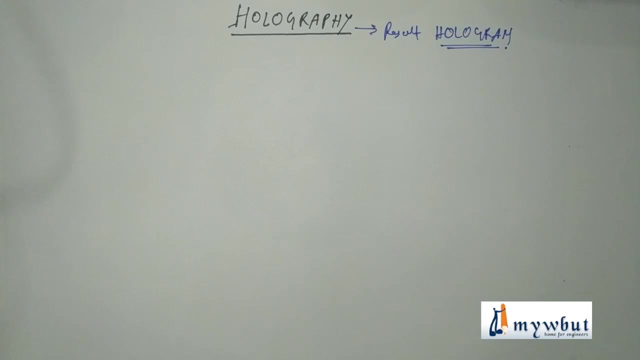 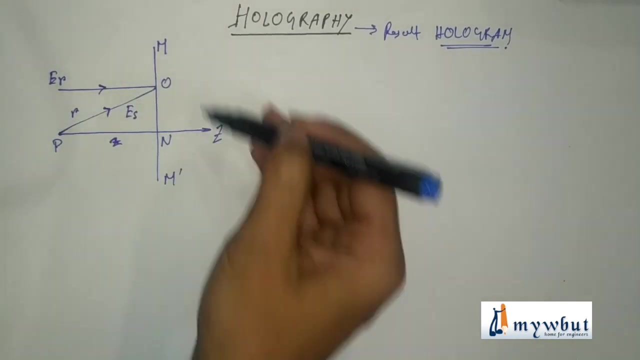 photograph is called a hologram, So the process is holography and the result is known as hologram. So now we will be explaining briefly the theory of holography. This is a schematic diagram, A very small diagram, of the working of the holographic process. So when a light beam, that is, 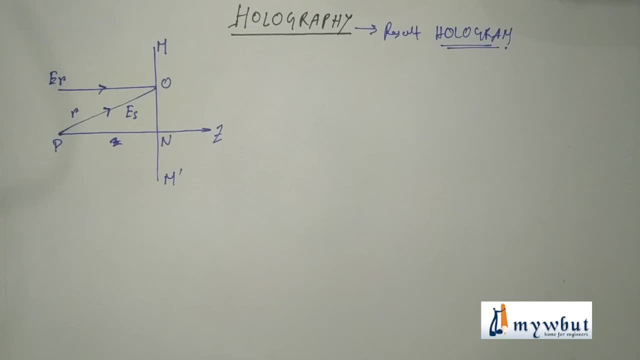 plane waves from a coherent source illuminates this small object. a part of the incident beam- that is the part of a plane waves- is scattered by the small object and produces spherical waves. The rest of the incident beams, that is, the reference beams, directly reaches at a photographic plate. 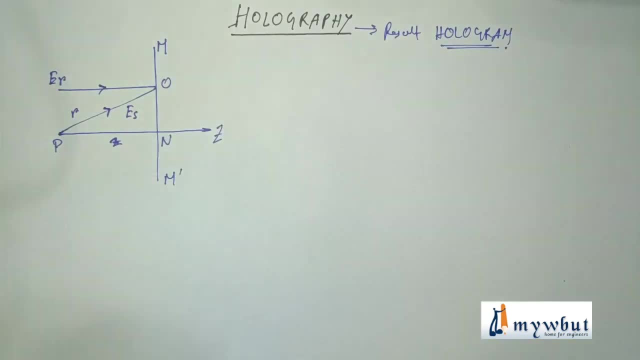 That is at this photographic plate. So this is the photographic plate that is at this photographic plate. In this way the reference beam and the spherical waves of the object beam reach at the photographic plate and interfere. That we have already studied before the process of interference To find the resultant intensity at O. that is, at this point. I 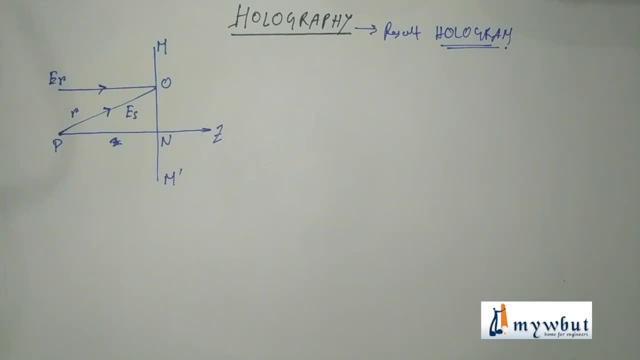 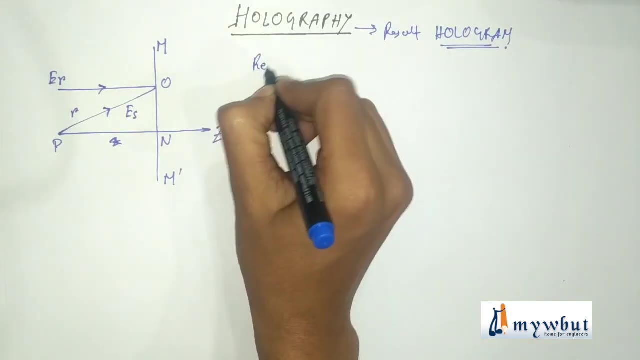 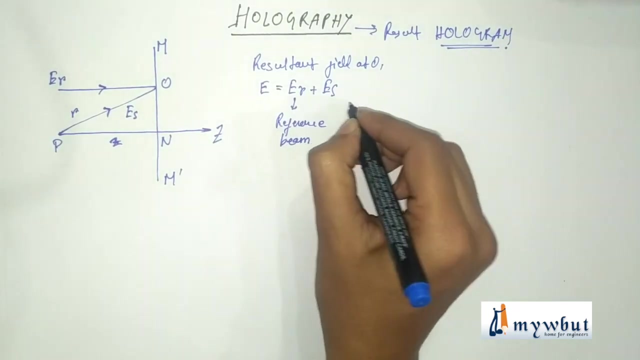 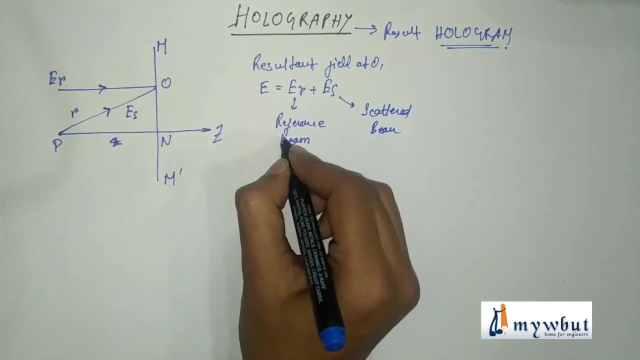 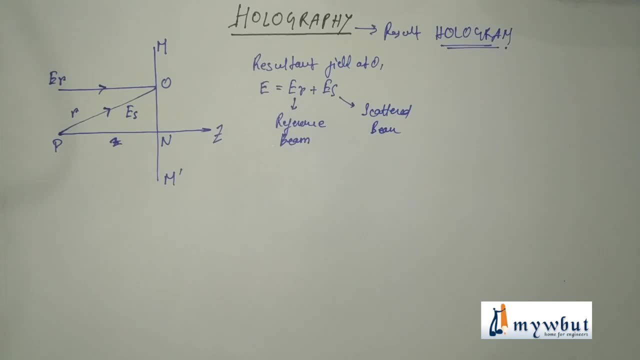 the reference beam is a plane wave, so we can write: ER is equal to ERO, e to the power, I into KZ minus Omega T, where Z equal to PN, that is equal to perpendicular distance of the object P from plate. in the scattered field, ES, both amplitude and phase vary with position. 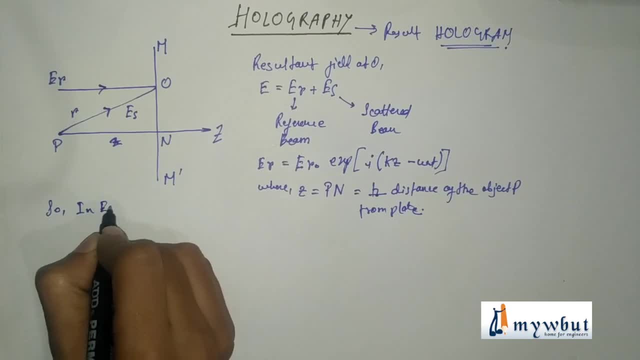 so in ES amplitude and phase vary with position. so in ES amplitude and phase vary with position. thus the scattered field can be given by ES that is equal to ESO, by R into e to the power I KR minus Omega T, where R equal to PO. so the total. 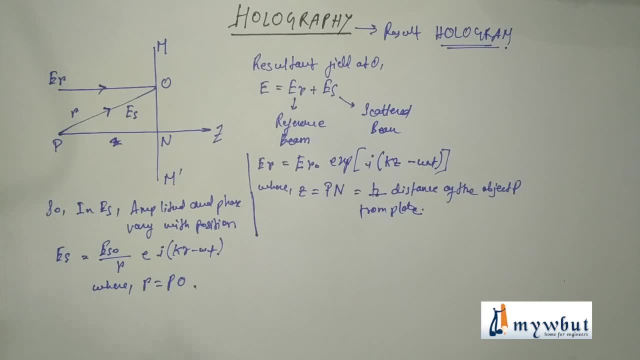 intensity at the point O on the hologram plate is given by. therefore, the total intensity at O will be given by I. that is equal to modulus of er plus es whole square. that is equal to er plus es into er plus es star. this is the complex conjugate of this value. so this is equal to er into er star. that is conjugate. 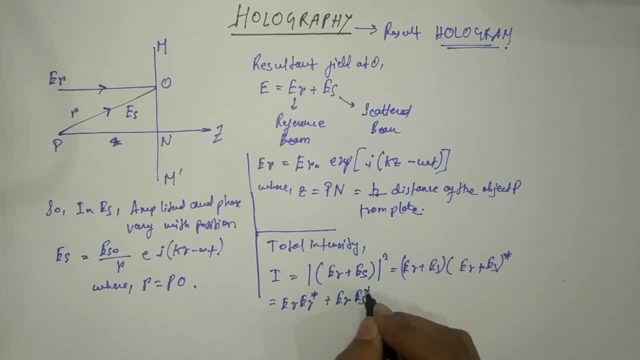 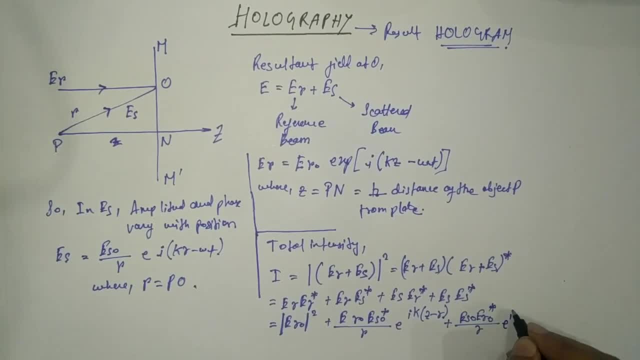 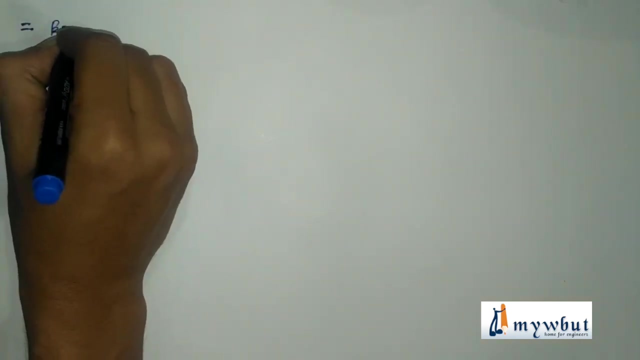 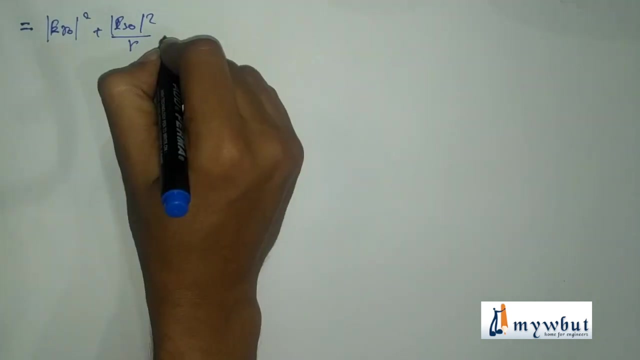 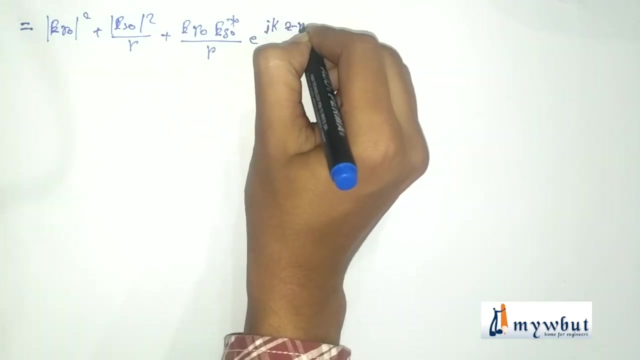 so, so, so e to the power ik r minus z plus eso. giving a modulus whole square by r square that will be equal to ero whole square plus eso. whole square by r plus ero into eso conjugate by r into e to the power ik z minus r plus. 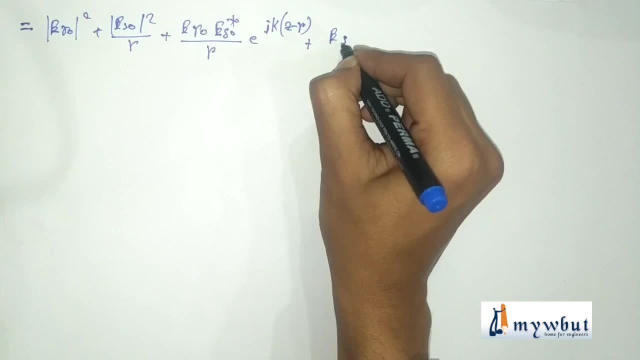 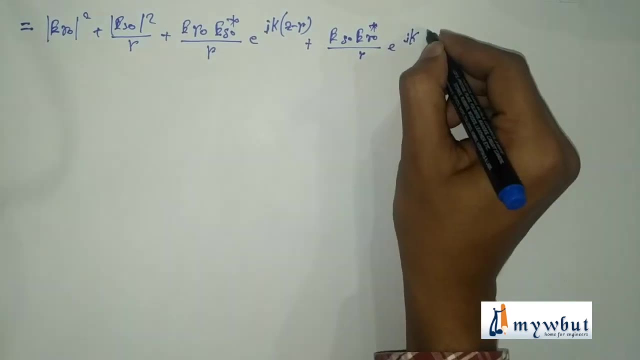 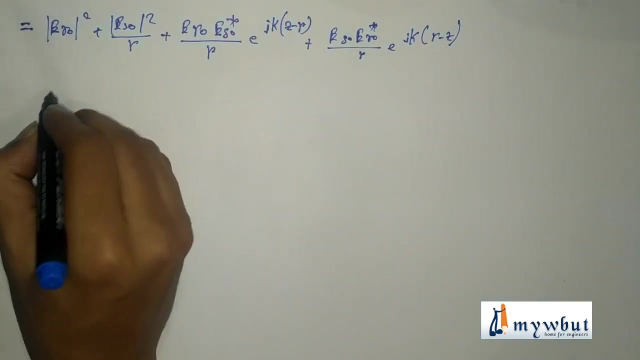 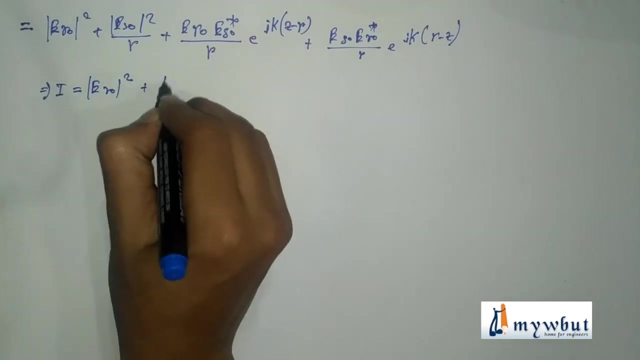 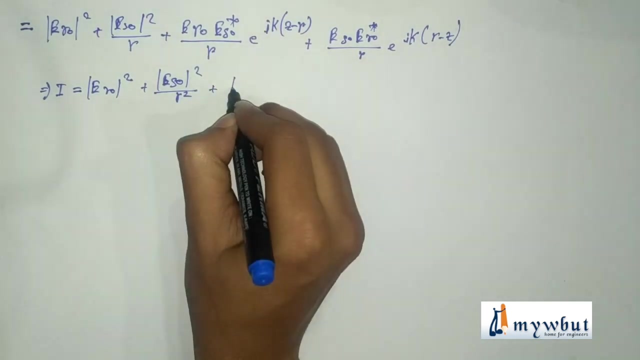 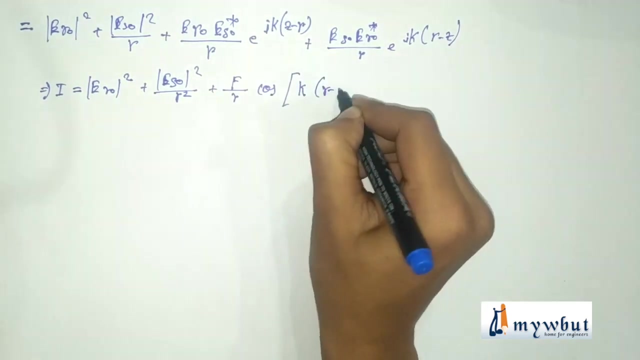 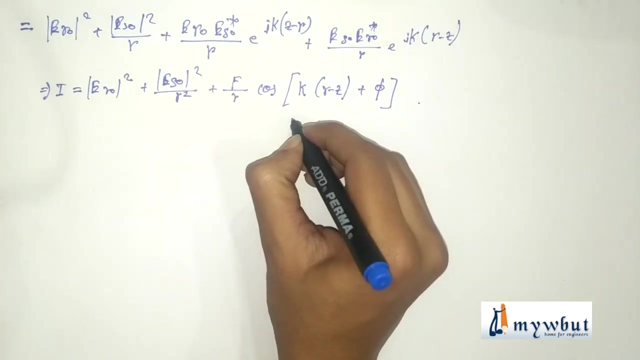 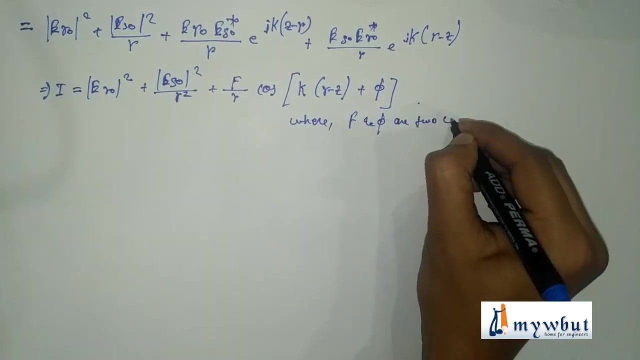 f by r cos of k into r minus z plus phi, where f and phi are two constants. this equation implies that intensity is a. 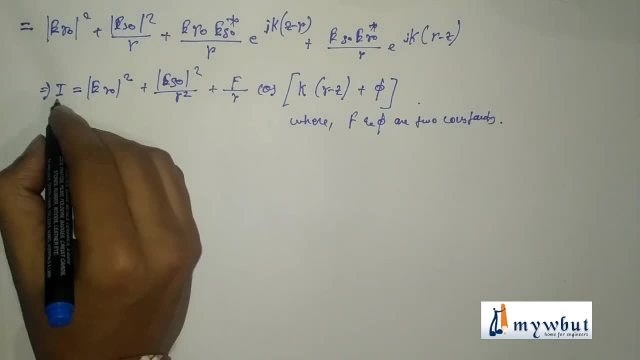 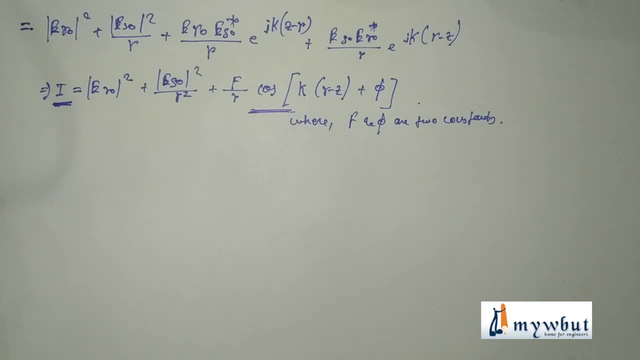 function of cosine term that you can see here. intensity is a function of cosine term. it implies that total intensity I passes through a series of maxima and minima due to its dependence on the cosine term. so it will depend on the value of cosine term for being a maxima and minima. now, if we assume the plate, 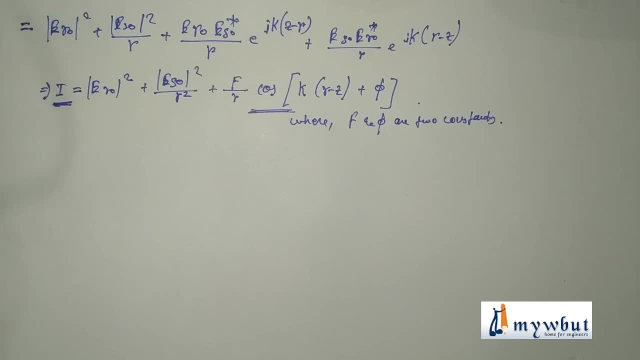 response varies with intensity. I, the power transmission coefficient of the plate, can be written as: the power transmission coefficient of the plate can be written as TP square, equal to 1 minus beta I, where beta is also a constant. now, since beta I is very, very less than 1, we can approximate the equation as TP. 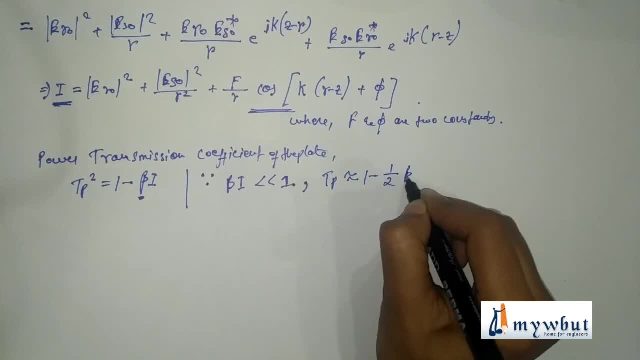 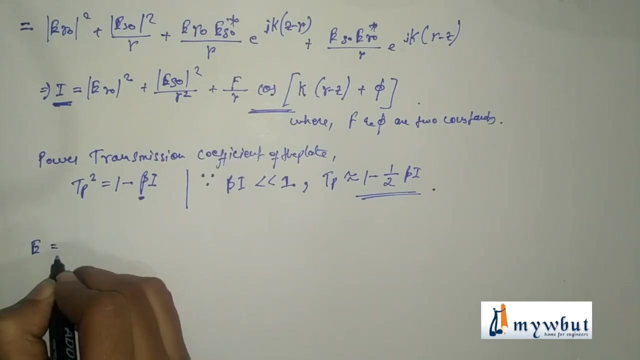 similar to 1 minus half beta I. so when the recorded hologram is illuminated by the reference beam, the field of transmitted wave E is equal to. I'm writing down the result of its one minus beta by 2 into E- ro whole square minus beta by 2 into ESO whole square by R square into E. of e to the